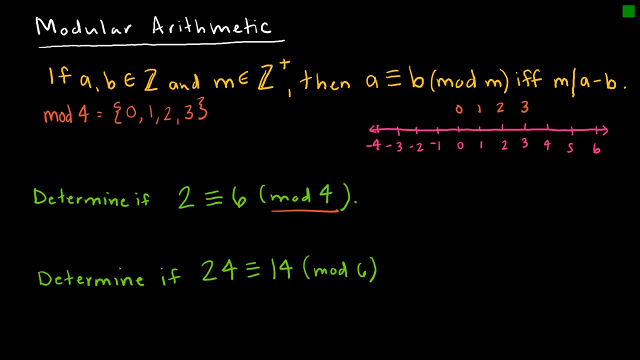 of 4,. 4 divided by 4 is a nice even number that has a remainder of 0, and 5 divided by 4 has a remainder of 1, and 6 divided by 4 has a remainder of 2, and similarly we could go in the opposite direction, where negative 1 would. 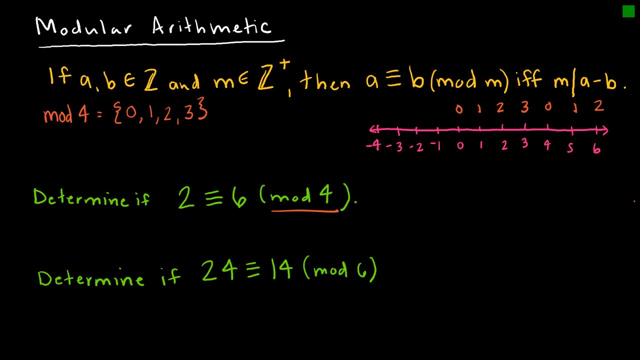 actually be negative: 4 divided by 4.. with a remainder of three and then two, and then one, and then zero, et cetera. So we can see what the pattern is is basically just zero, one, two, three. 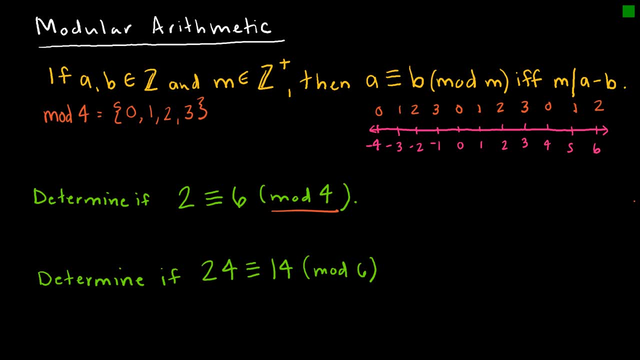 zero one, two, three, zero, one, two, three, et cetera. So what we're looking for in our first example asks us, is two congruent to six in the world of mod four. So looking at mod four, two and six. 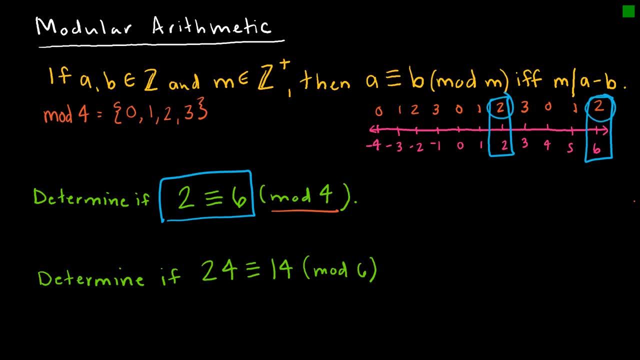 if you'll notice, both are two, which means if I take two divided by four or six divided by four, my remainder is two, exactly the same. So that's good. so that means, yes, they are equivalent. Now, what I want to do instead is look at my definition. 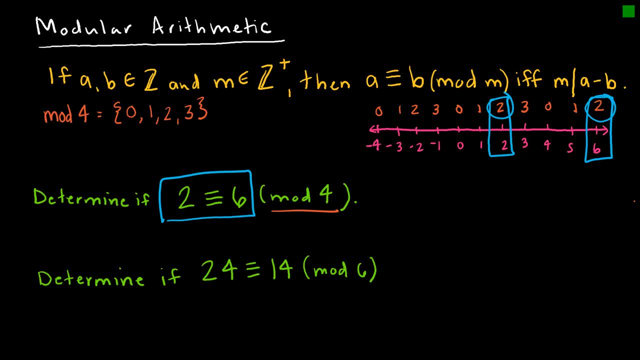 Now my definition says: I can determine that without making a number line and counting everything out by saying: is the difference between these two values divisible by four? And that is what we're asking here. So we're saying: does four divide two minus six? 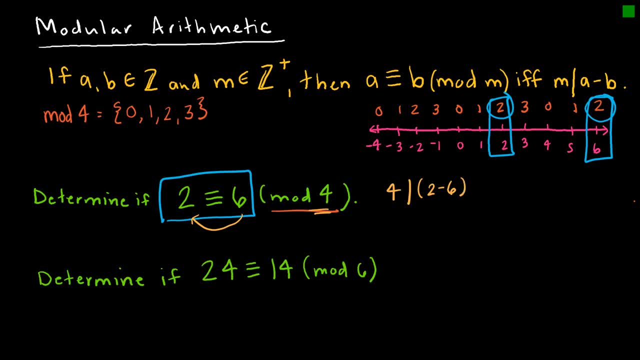 or six minus two would give us the same result. So does four divide negative four, And four does divide negative four, and therefore we know that, yes, two is congruent to six. So we're not saying that two is divisible by four. 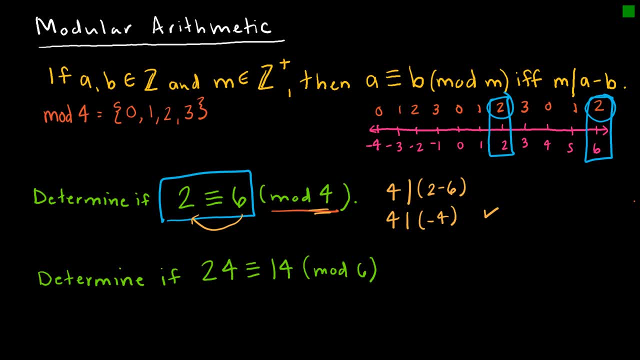 or that six is divisible by four, but that these two are equivalent because the differences in their remainders is divisible by four. So let's look at our next one: 24, is 24 congruent to 14 mod six. So again we're asking: does six divide 24 minus 14?? 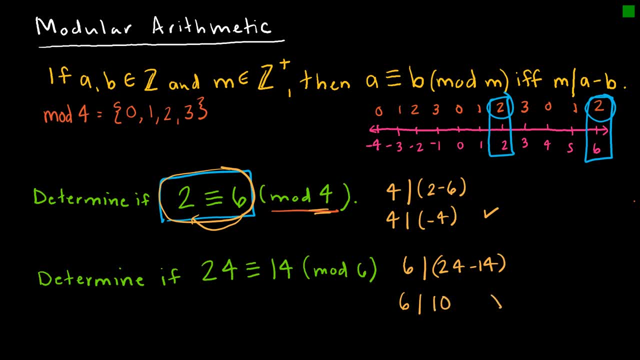 Does six divide 10?? And in this case six does not divide 10 evenly and therefore no, these are not equivalent. Again, we could draw out a number line and we could see that visually. but hopefully you get the basic idea of modular arithmetic. 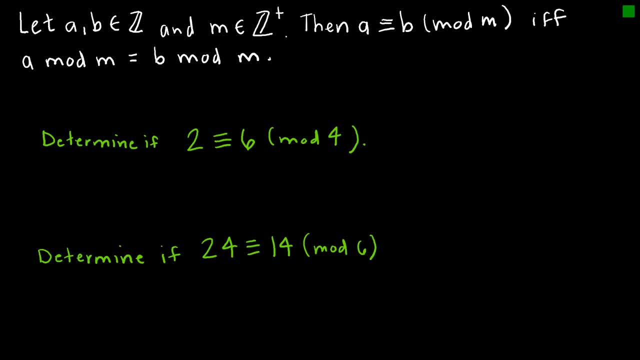 We've just looked at the definition of modular arithmetic and I want to look at a theorem that really follows from that And I feel like this theorem is pretty straightforward. Essentially it's saying all the same things we had before: a mean integers, m is a positive integer. 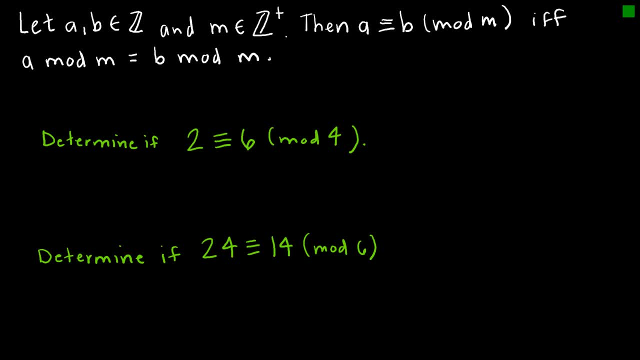 then a is congruent to b mod m, if and only if, and then a mod m is equal to b mod m. So really all we're saying is, if the remainders are equal to one another, then they are congruent. 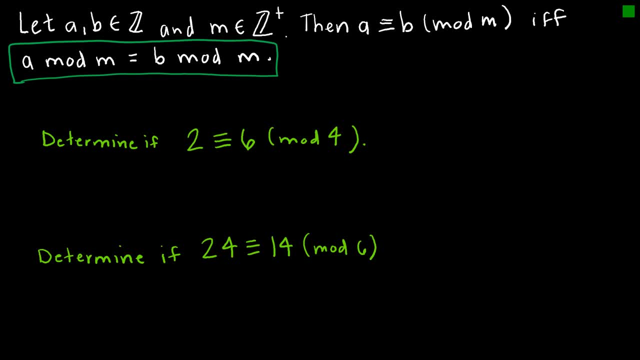 And that's what we talked about when we looked at our last slide. but let's kind of look at it in terms of the mathematics. So I put the same two examples that we had earlier, but I'm going to add on the last slide. 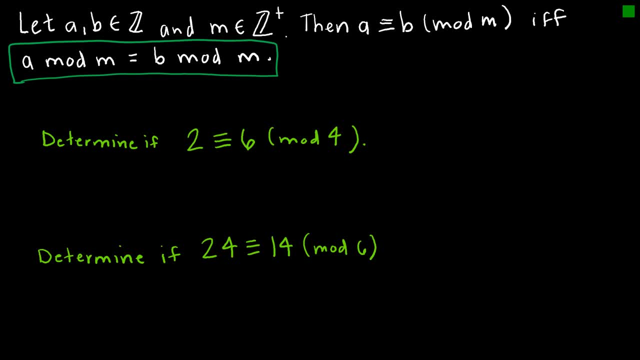 And I just want to look at it in terms of when we looked at the division algorithm. So if I'm looking at two, I'm saying: does four divide two? And again we know the way that we can write this- We're saying four times some number. 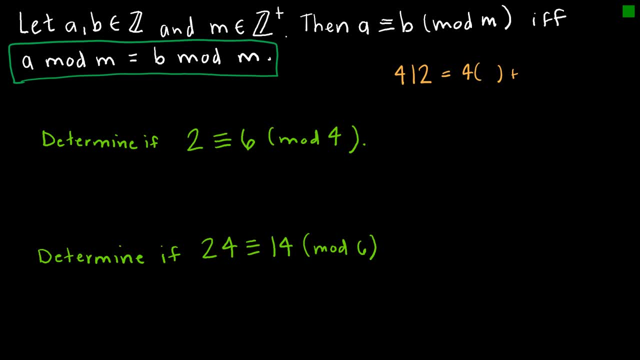 plus some number equals two. That's what we want to look for. So in this case, four times zero plus two does equal two. To write that in terms of r, which is the remainder, the remainder is equal to two mod four. 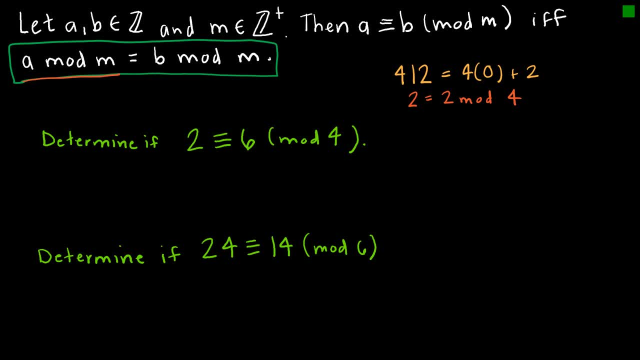 So two mod four. So notice what I'm building up to here: a mod m- I'm saying two- is equal to two mod four. Let's look at six. So does two divide six? Sorry, let me try that again. Does four divide six? 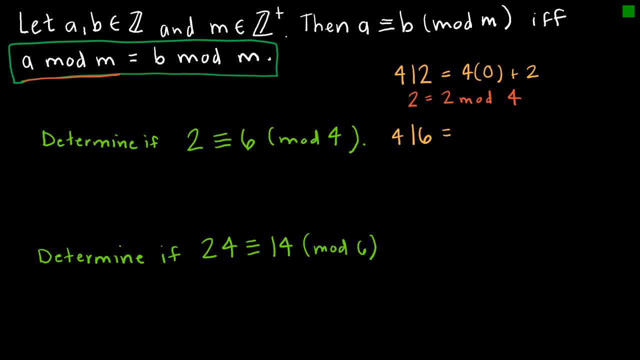 I got confused for a minute, And so again, the way that we would write that is four times some number plus some number, using the definition of division, And in this case we would say: four times one is four plus two is six, And again the remainder of two would be equal to six. 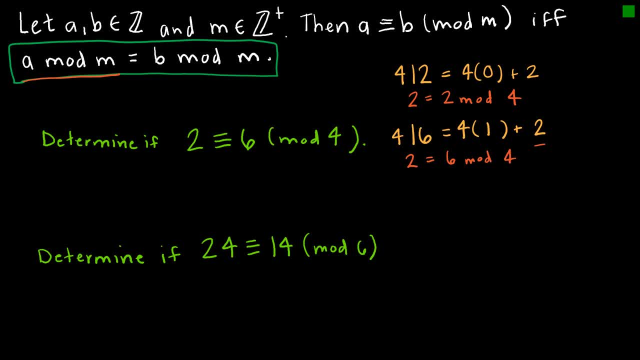 So two times two is equal to six mod four. And so, notice, what I've just shown you is that, yes, in fact we already knew these were equivalent, but now I'm just showing you in another way that two is equal to two mod four. 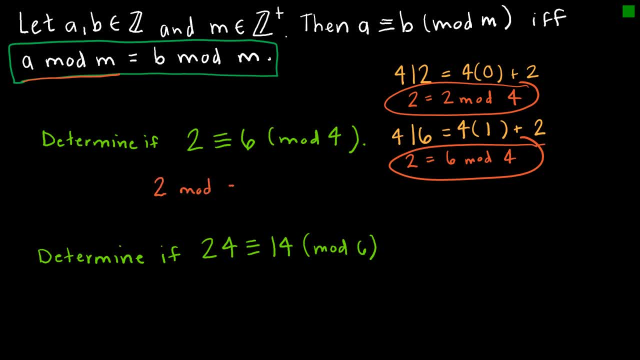 two is equal to six mod four and therefore two mod four is equal to six mod four And therefore we can say, yes, this is true. Let's look at our other example And again, we previously showed that this was not congruent. 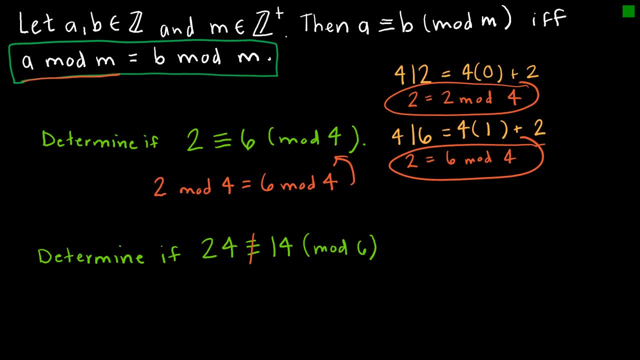 So let's take a look at how we might show that mathematically. So we're saying: does six divide 24?? And if we take six divided by 24, we're saying six times some number plus some number is equal to 24.. 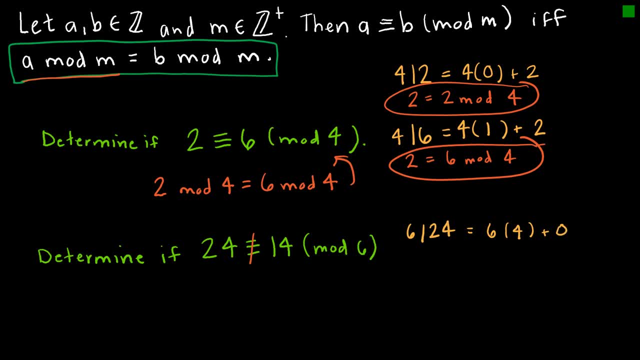 In this case, six times four is 24 plus zero. So how would I write that? I would say that my remainder of zero is equal to 24 mod six. And now let's look at the other one. We have 14.. 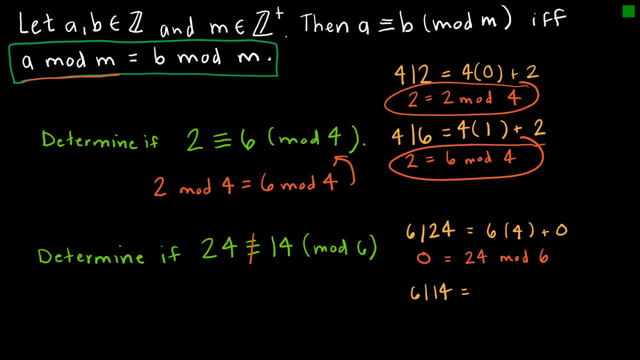 So does six divide 14?? And again we're saying: six times some number plus some other number, This one would be six times two is 12 plus two is 14.. And notice here, my remainder is two. So two equals 14 mod six. 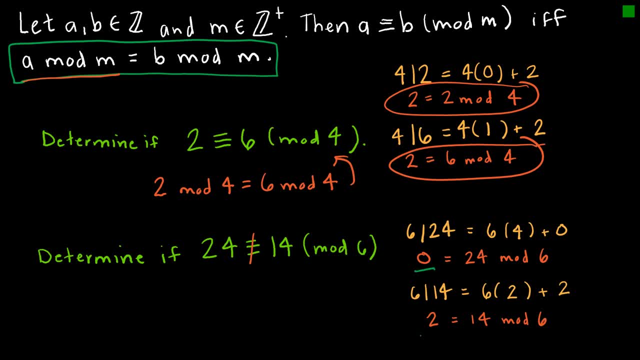 And obviously these values are not equal. Therefore, 24 mod six does not equal 14 mod six And therefore we can say again that 24 is not congruent to 14 mod six, Now that we have a basic framework for modular arithmetic. 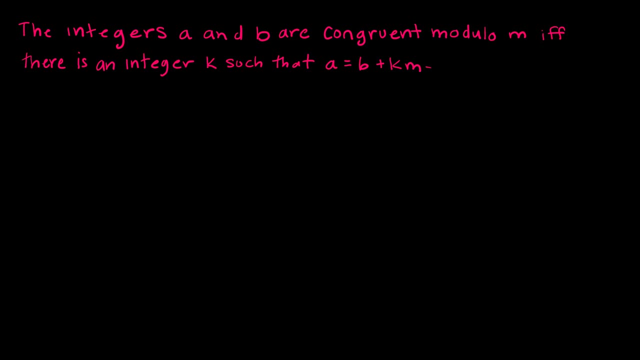 I want to look at a few theorems and their proofs before we do any actual computation. So the first theorem says: the integers a and b are congruent. modulo m, which is just a, is congruent to b mod m. And then we have this if, and only if, word. 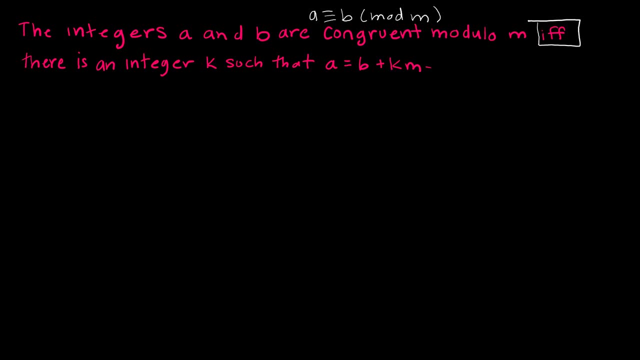 And keep in mind whenever we have if and only if. that means you have to prove it in both ways. That means you have to prove it in both directions. So assume this, prove this and then vice versa. And what am I trying to prove? 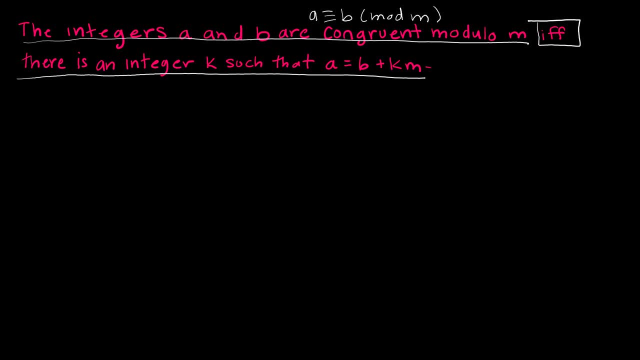 There is an integer k, such that a is equal to b plus km. So notice, here I'm going from congruence to an equation. So let's start by assuming a is congruent to b mod m. So I'm assuming we'll call this p proving q. 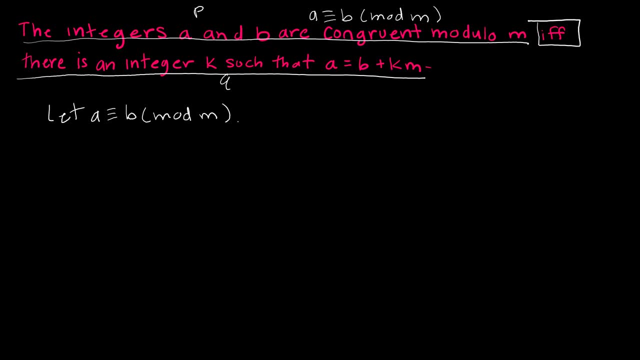 So let a be congruent to b mod m. What do I know about? when things are congruent? Well, based on what we've learned in this video, then we can say that m divides a minus b. Why can I say that? 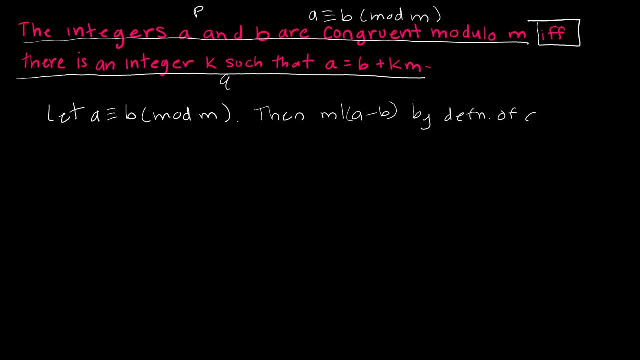 By the definitions of congruence. Now, if m divides a minus b, then I can say that a minus b is equal to km for some integer k. And again, how do I know that? By definition of divisibility. Now think about where I'm trying to get to. 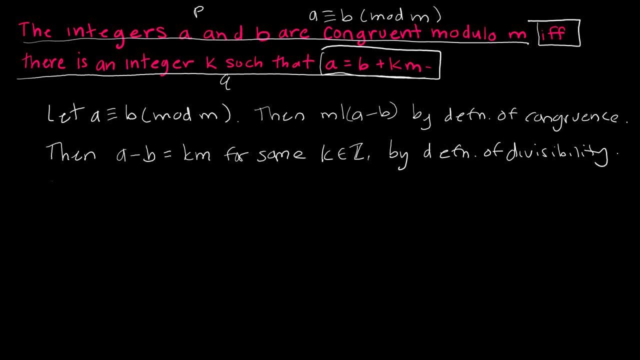 a is equal to b plus km. I'm really close here By addition, or you can even be specific by addition of b, because I'm going to add b to each side, then a is equal to b plus km. So I've shown that if p is q, then q must be true. 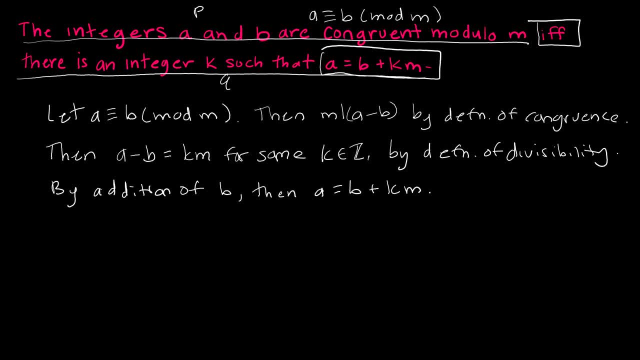 Now I have to show: if q then p, So assume a is equal to b plus km, Then a minus b is equal to km by subtraction. And as you can see, I'm just kind of going in the reverse order, But what I have to show then 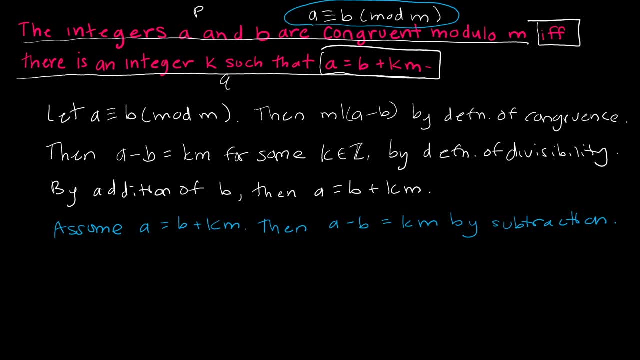 is that this is true. So if a minus b is equal to km by subtraction, what does that tell me? That tells me that m divides a minus b, so a is congruent to b mod m. And again I didn't give the reasons for each step there. 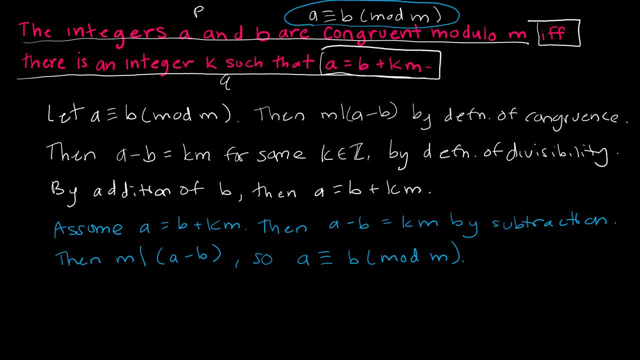 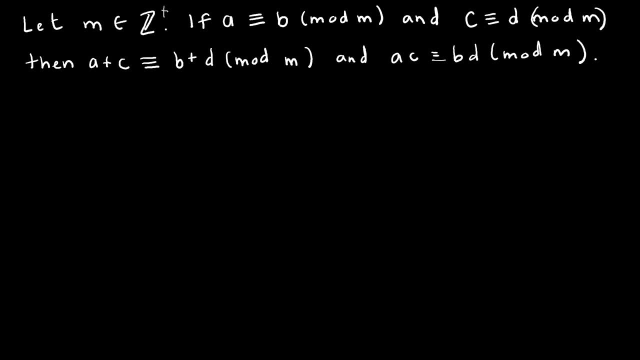 just because I was going. I'm using the same reasons as I did in the proof above, So I've proved this one in both directions. Let's take a look at another theorem now, and we're actually going to use the last theorem that we proved. 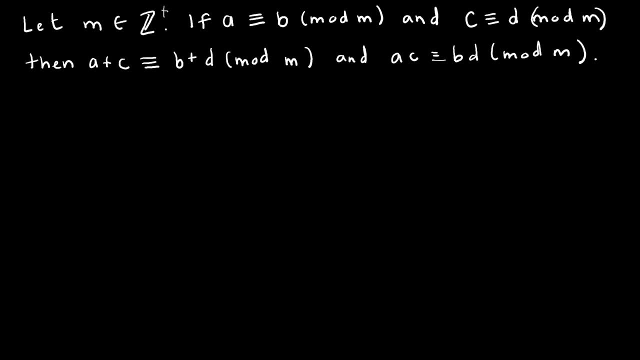 to help us prove this. So this theorem says: let m be some positive integer: if a is congruent to b mod m and c is congruent to d mod m, then a plus c is congruent to b plus d mod m. 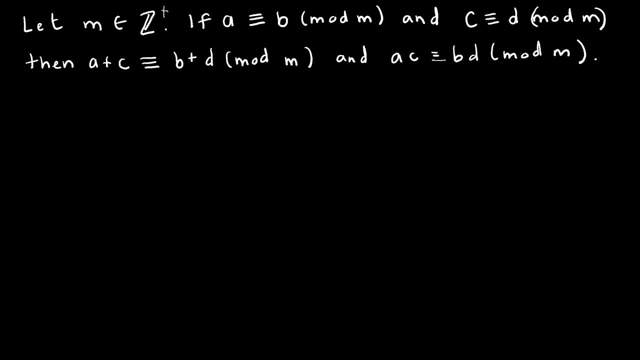 and a times c is congruent to b times d mod m. So again, this is not an if and only if statement, it's just an if-then. so it's just a one-direction proof. But there's two parts. I have to prove that this is true. 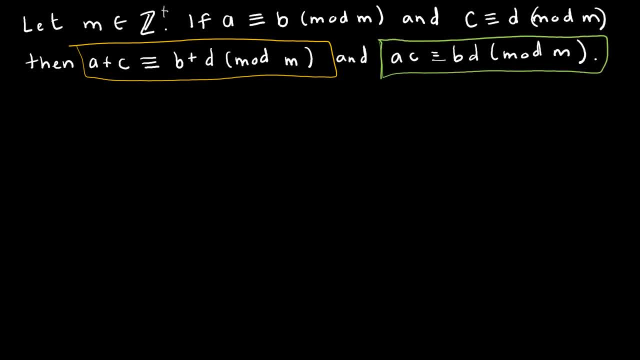 and I have to prove that this is true. So, before I prove either of those things, let's give ourselves some assumptions. We're going to assume, and again, if I wrote this as a proposition, it would be if: blah, blah, blah, blah, blah. 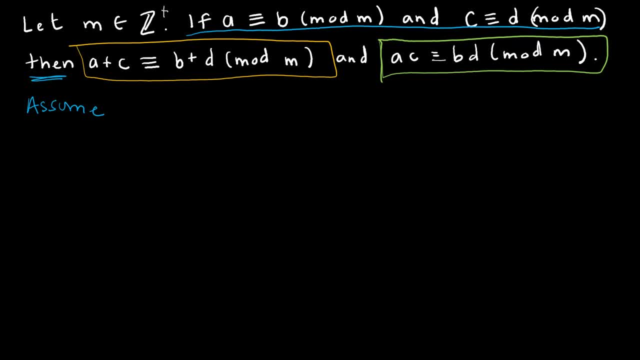 then, and so I'm assuming the if part. So assume a is congruent to b mod m, then what does it mean to be congruent? Then I can say that a is equal to b plus km for some integer k. Assume also c is congruent to d mod m. 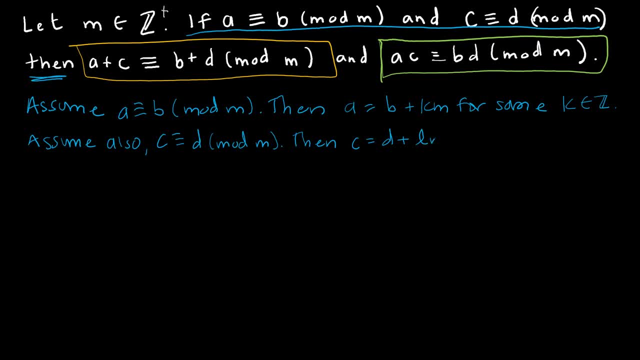 then c is equal to d plus lm. for some l, that is an integer. So I'm just going to use those as assumptions for each of the two parts of the proof that I'm going to go about proving. So I'm going to start with a plus c. 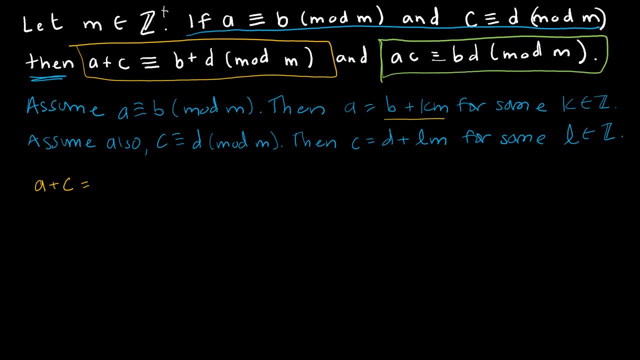 By substitution: instead of a, I'm going to plug in b plus km, And instead of c, I'm going to plug in d plus lm. From here, I'm going to just do some rearranging. I'm going to use both the associative. 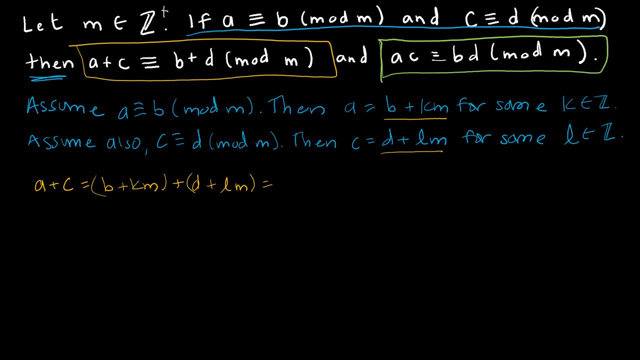 and commutative properties and I'm not going to write down each step, I'm just telling you the steps as I go. I'm going to use both the commutative and associative properties to rewrite this as b plus d plus km plus lm. 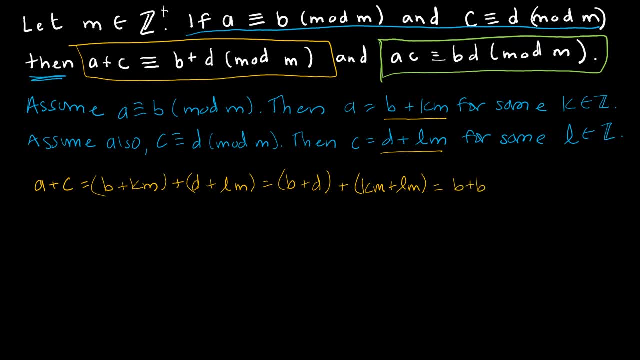 And then by the distributive property, I'm going to call that b plus d equals m. I'm sorry, not equals b plus d plus m times k plus l. Now, what am I trying to prove? I'm trying to prove that these things 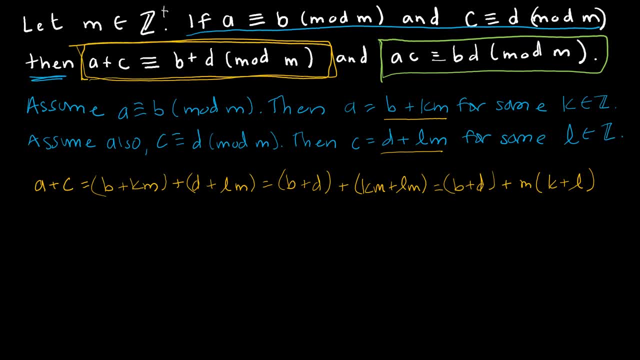 are congruent. modulo m, which means- right now I have a plus c- is equal to b plus d plus m, k plus l. So a plus c minus b plus d is equal to m times k plus l. And what does this mean If we have m times k plus l? 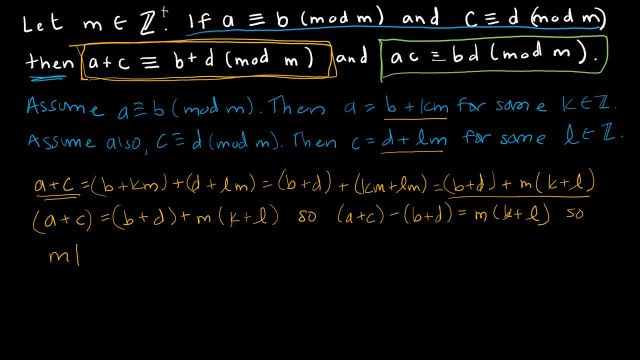 so m divides a plus c minus b plus d. So a plus c is congruent to b plus d, mod m. So a lot like that last proof that we did. I need to show that m divides it and therefore that they are congruent. 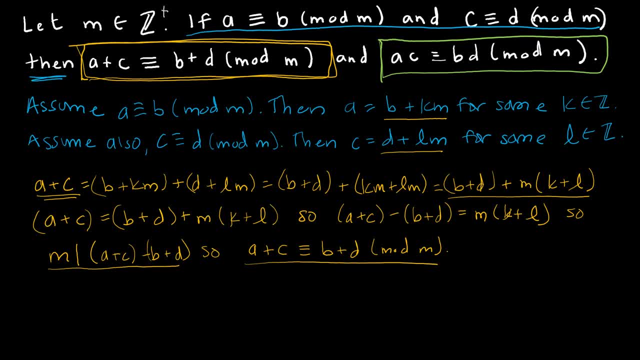 So I'm just using a lot of definitions. I apologize, I didn't write down the reasoning for each of those steps, but I feel confident that you can look at our last example and write down those yourself. I'm just dealing with limits, I'm just dealing with limited space here. 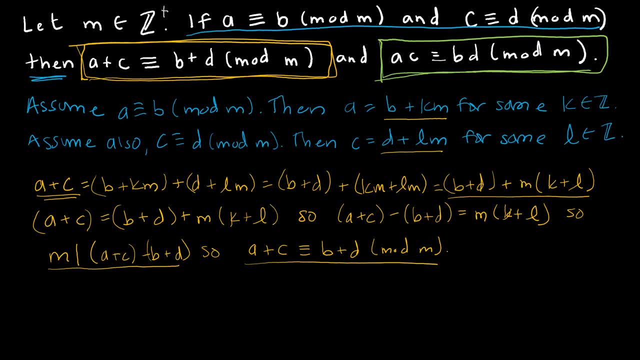 So now let's do the exact same thing. I have a times c is congruent to b times d mod m. So I have to take a times c, And a times c would be by substitution b plus km, times d plus lm, And again I can do some math. 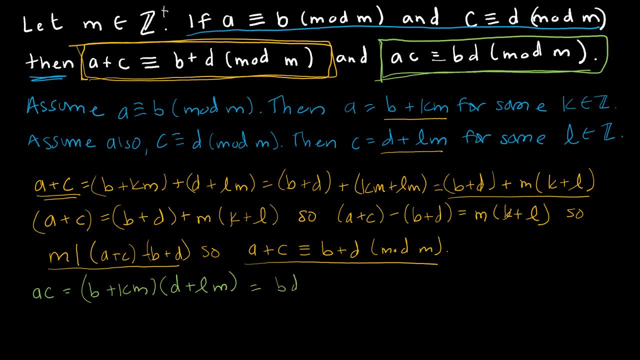 Some distributive properties. So I have bd plus blm, not d, blm plus kdm plus klm. That's horrible handwriting, klm squared, And really I'm just trying to write this kind of in the same way that I did the last one. 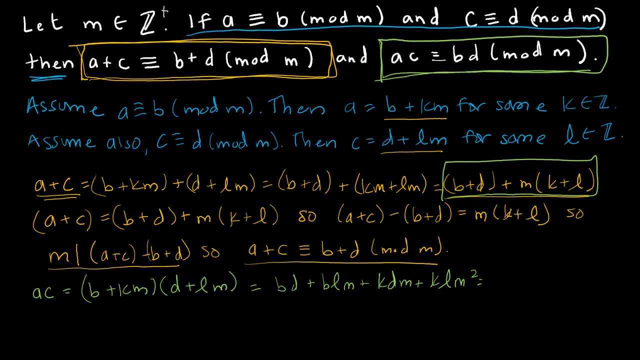 So can I do? that is the question. Well, I can say that this is bd plus m times vl, plus kd plus klm. So what does that tell me? So a times c minus b times d is equal to m times all of that. 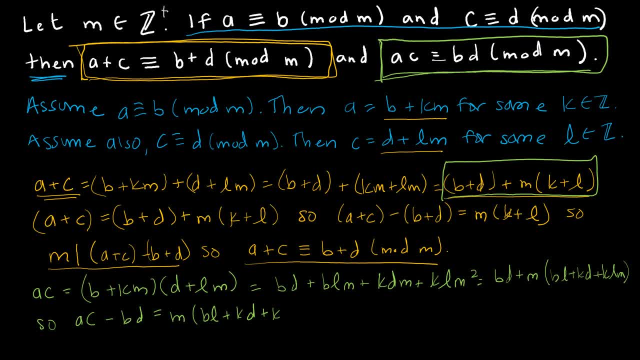 vl plus kd plus klm. And again, if I can do that subtraction and that subtraction results in m times something, then m divides all of that. So m divides ac minus bd. So ac is congruent to bd mod m. Let's take a look now at those same theorems again. 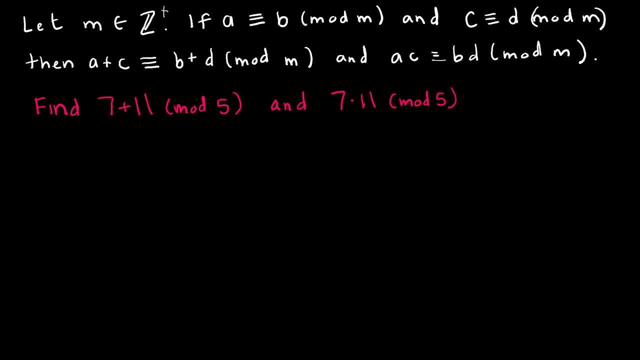 and actually use them in an example. Before we actually use those theorems, though, I want to look at just some regular modular arithmetic with you. So this one says: let's find 7 plus 11 mod 5.. If I were to find 7 plus 11 mod 5,, 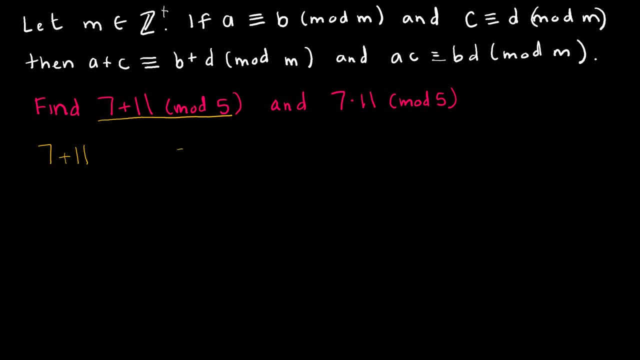 then really what I'm going to do is take 7 plus 11 to get 18.. And then say 18 is congruent to, so it's not equal to, but it's congruent to. And then I'm going to think about if I took 5 into 18,. 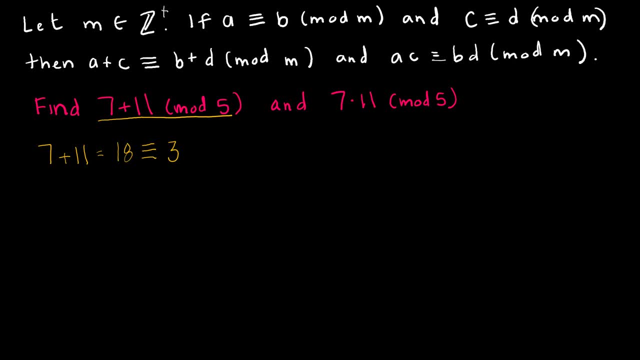 what's my remainder? And the remainder would be 3, because it goes into 15 evenly, with 3 left over, So 3 mod 5.. So again notice, I switched from equals to congruent, to Now let's take a look at the theorem. 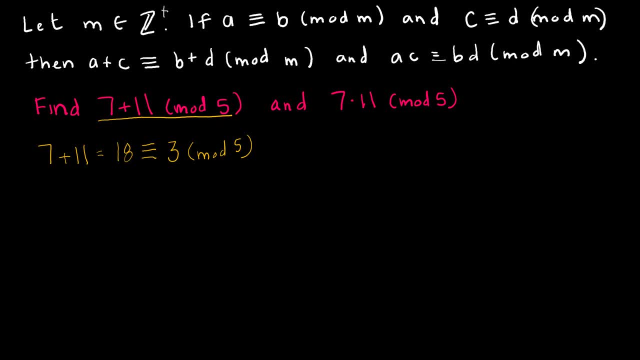 The theorem says: if a is congruent to b, mod m. so essentially they're saying: let's take a look at 7.. What is 7 congruent to mod 5?? Well, if I took 5 into 7, that would be a remainder of 2.. 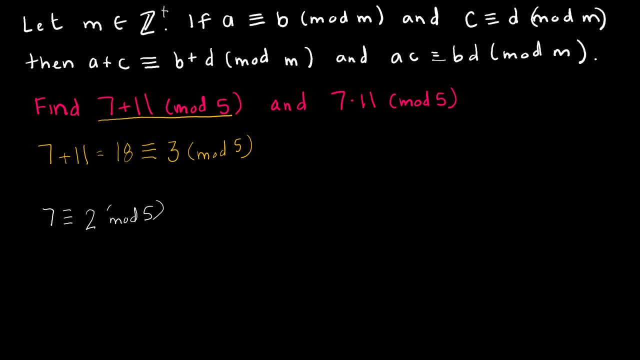 So 2 mod 5.. And 11 would be congruent to 1 mod 5.. So if I wanted to do this question again, 7 plus 11 would be congruent to 2 plus 1 mod 5, which would be equal to 3 mod 5.. 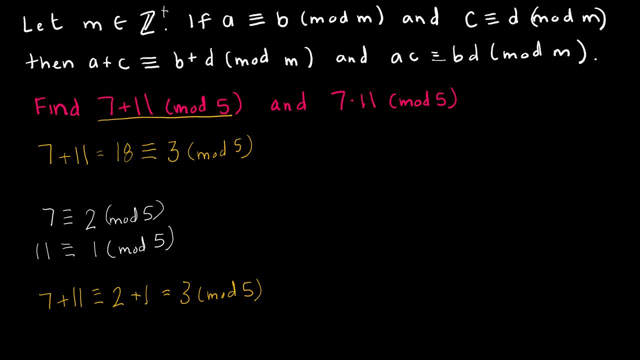 Now let's take a look at our other practice. We have 7 times 11.. So, again without our theorem, 7 times 11 would be 77, which would be congruent to 2 mod 5.. Again, using what we learned here, 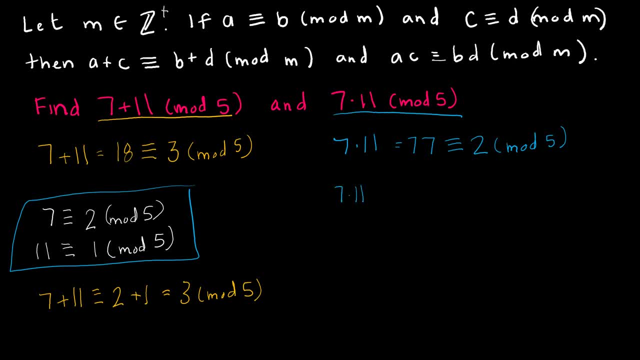 we could also say that 7 times 11 is congruent to 2 times 1, which is equal to 2 mod 5.. So, again, not a proof. We've already done the proof. This is just showing how those theorems might be used in an actual example. 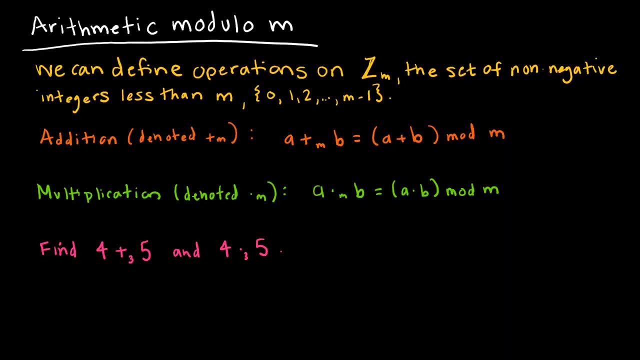 I also want to point out to you some different notation that you might see. So we already sort of did an example: 7 plus 11 and 7 times 11.. And I didn't use this notation just because I didn't want to throw something else new in there.